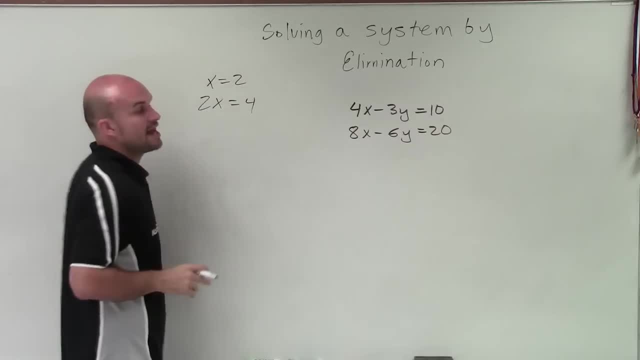 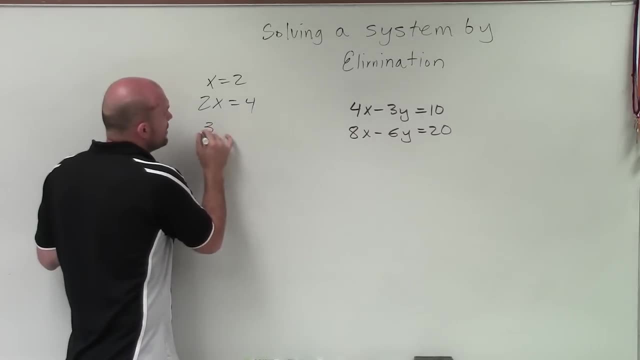 be: 2x equals 4.. Now notice on the left and to the right: I multiplied by 2.. But is 2x equal to 4? the exact same thing as x equals 2?? Yes, it is. What about if I multiply by 3x? Is 3x equal to 6? 3x equals 6, is that the exact same? 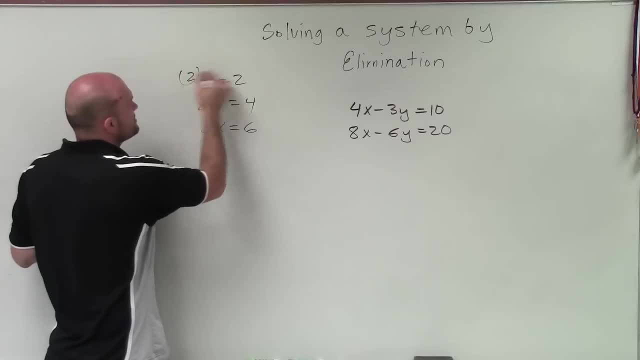 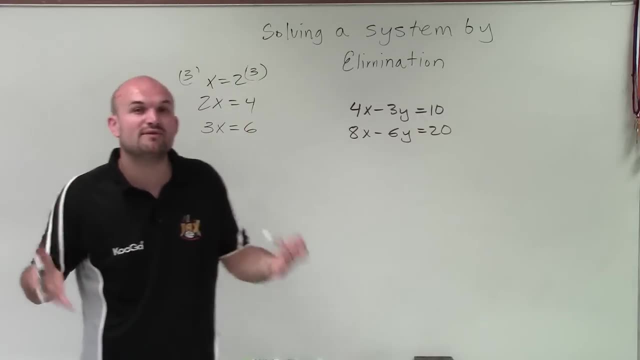 thing as x equals 2?? Yes, And all I did for each one of these terms is I just multiplied by a multiple, by either multiplying by 2 or multiplying by 3.. So you can keep equivalent equations if we multiply by a multiplier. 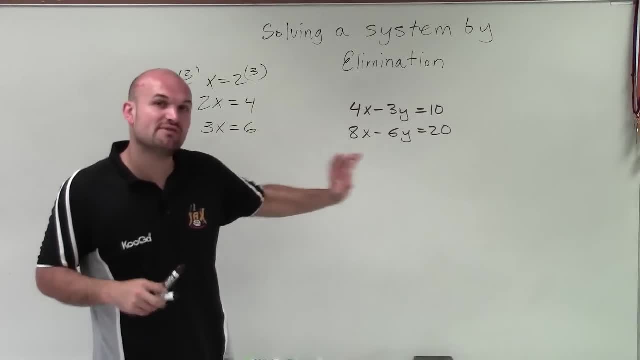 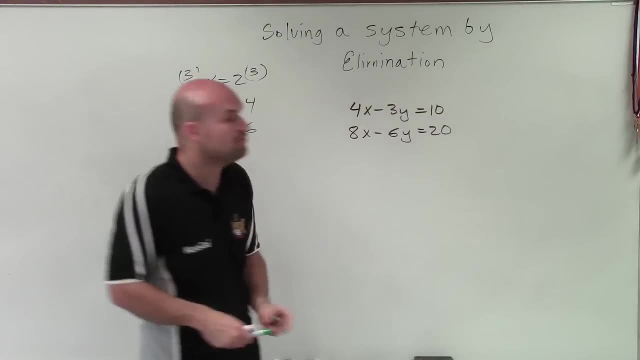 So what I want to do is I need to create an equivalent equation that's going to have the exact same coefficient for one of my variables, And I chose to have the same variable as x, So we can multiply by a multiplier. Now we can multiply either way. We can multiply. 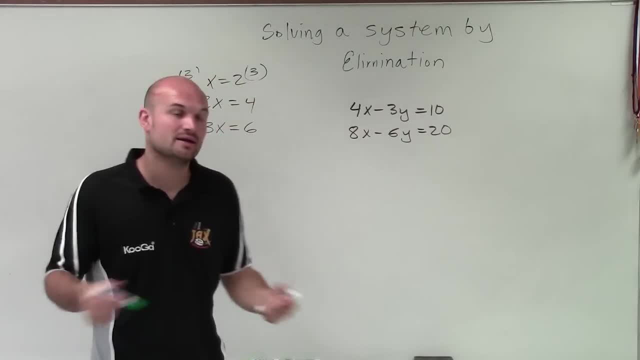 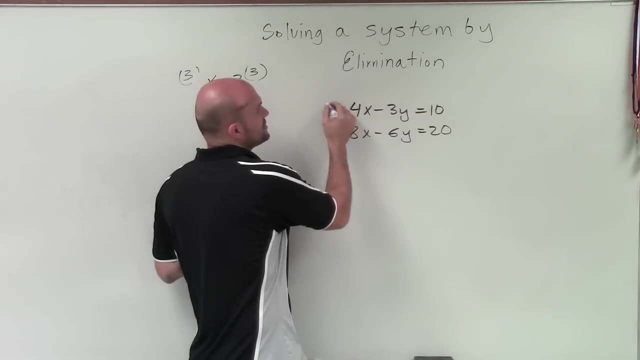 by fractions, which most people don't like to do, or we can multiply by our integers. So if I want to get 4 and 8 together, I need to look at what is the least common multiple between 4 and 8, which in this case is going to be 2.. I'll be right back over, So in this, 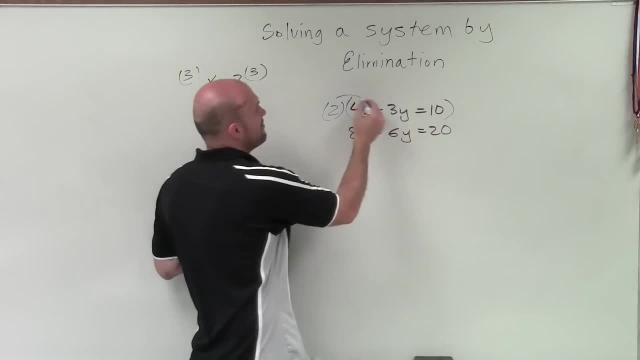 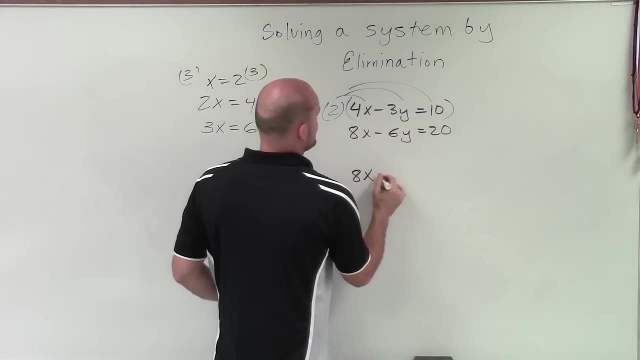 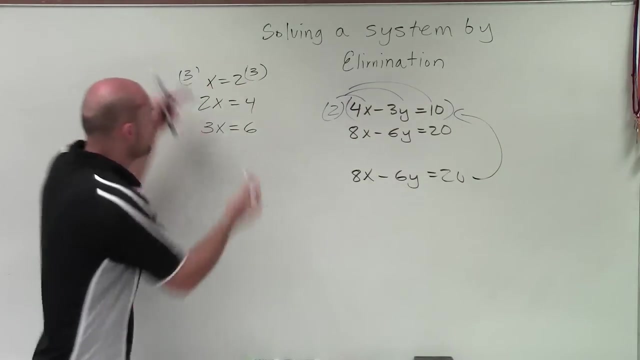 case, it's going to be 2.. So now, by looking at this, when I multiply my multiplier, now I'm going to create a whole brand new system of equations which is going to be: x equals 8x minus 6y equals 20.. This equation is exactly the same as that equation, It's just like. 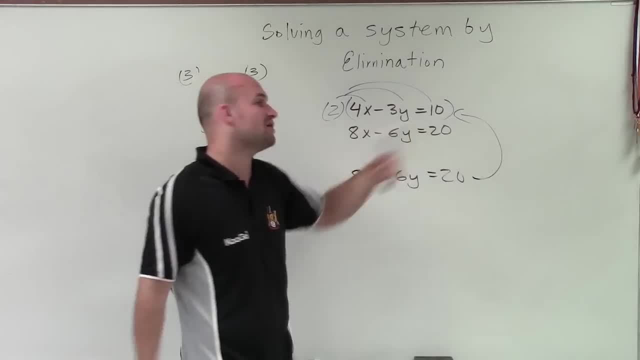 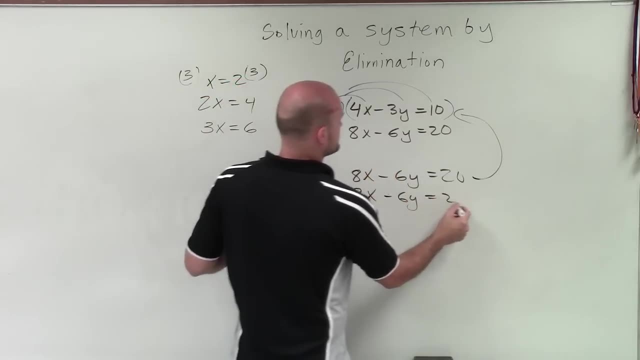 x equals 2 and 2x equals 4.. It's the exact same. It's just being multiplied by a multiplier. So now I have 8x minus 6y equals 20.. And what you notice is these are exactly the same equations. 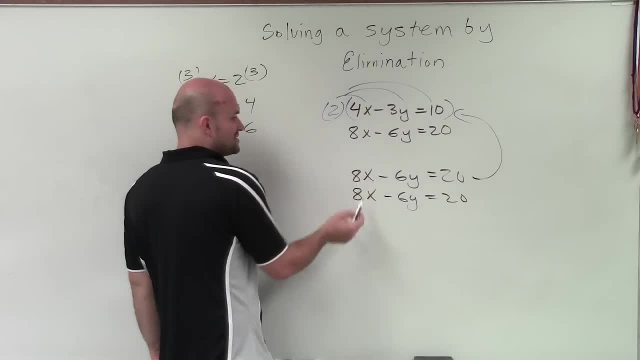 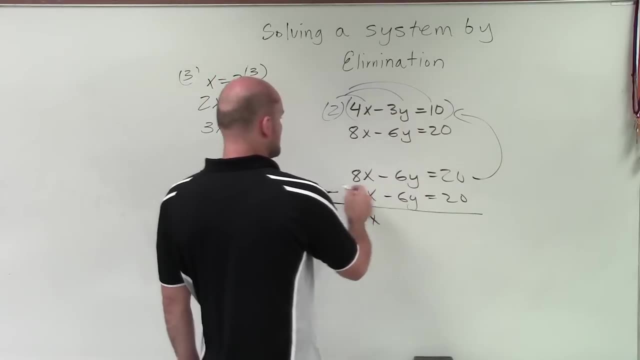 exactly the same equations. So if I go ahead and do my subtraction saying I want to eliminate the 8x and the 8x subtract, I get 0x negative, 6x plus. so I get a positive 0y equals 0. So I get 0 equals 0. Well, 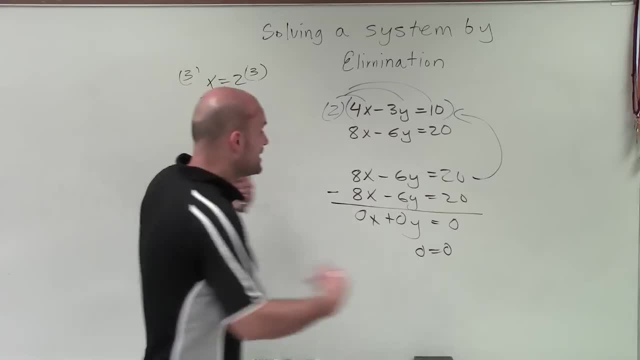 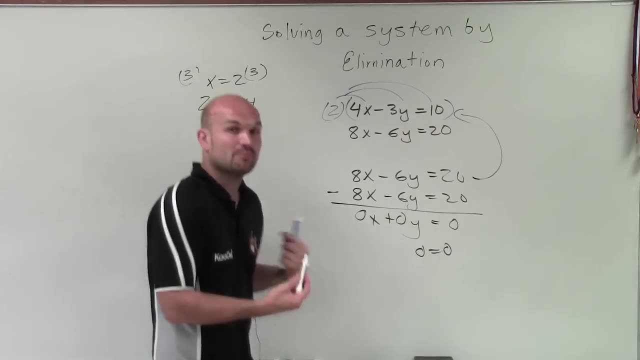 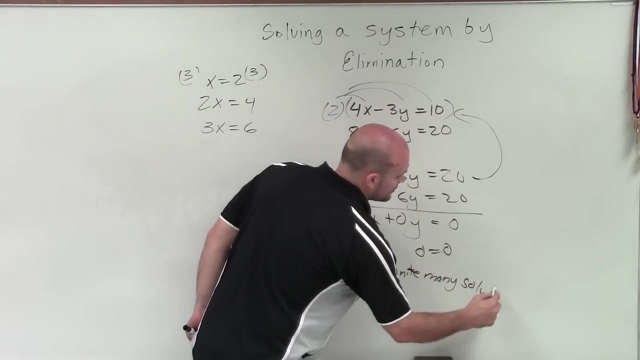 now, I don't have a value of x, I can't find a value of y, But I know, when I eliminated my x, I ended up eliminating my y, But I got a statement that was true. So therefore, the number of solutions is going to be infinite. many solutions. So there you go, ladies and